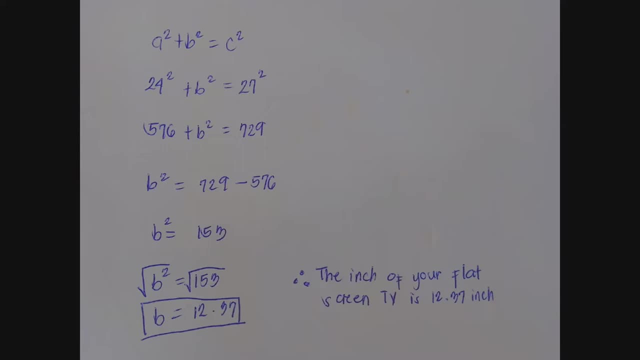 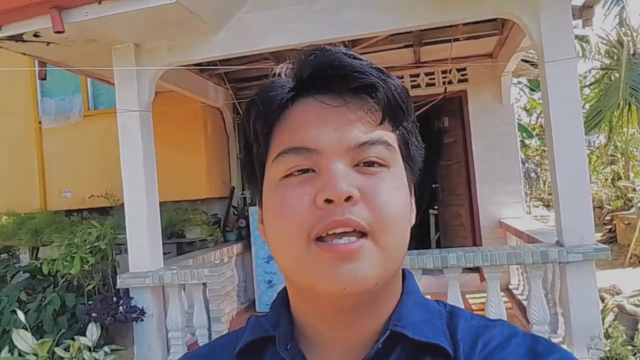 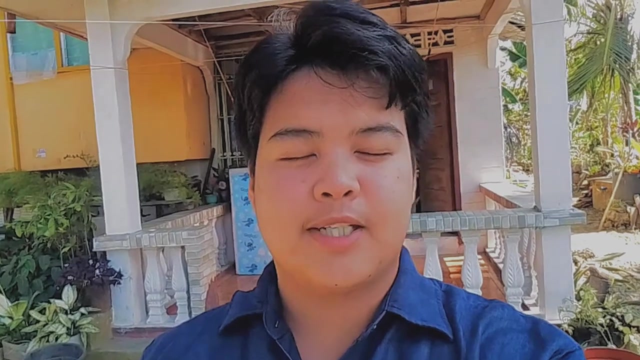 So, therefore, the inch of your flat screen TV is 12.37 inches. So for the second examples of Pythagorean theorem on real life, situation is finding the measure of the beam of our house, Because my mother want to change it because it's too old, and we need to find the measure of the beam of our house. 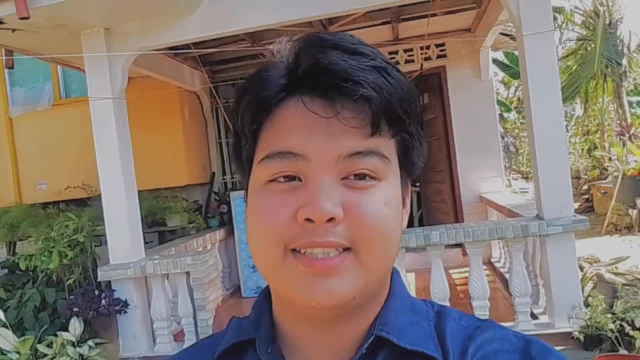 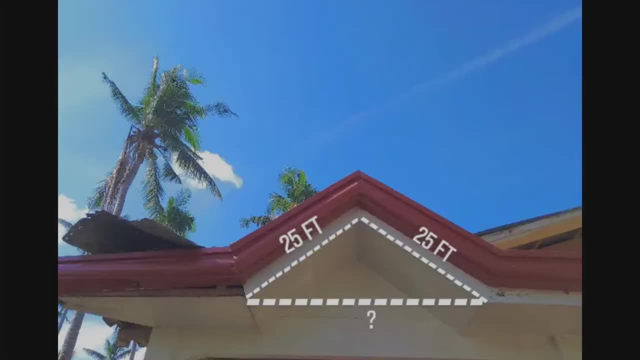 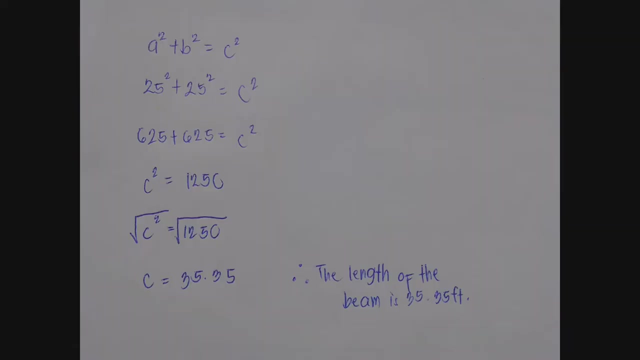 So to find the measure in order to buy the exact materials that we needed to change into a new one. So this is the image for our second examples of Pythagorean theorem on real life situation. So this is our solution for our second examples of Pythagorean theorem on real life situation. 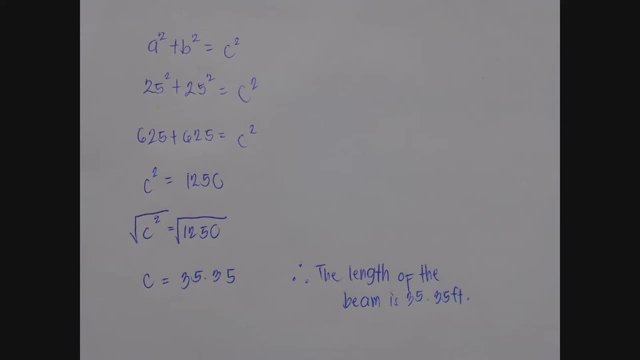 Using the formula: a squared plus b squared equals c squared. So first we need to substitute the variables, So we are going to multiply. So A equals to 25, B is equal to 25, and C is the unknown Square root. 25 is 625.. 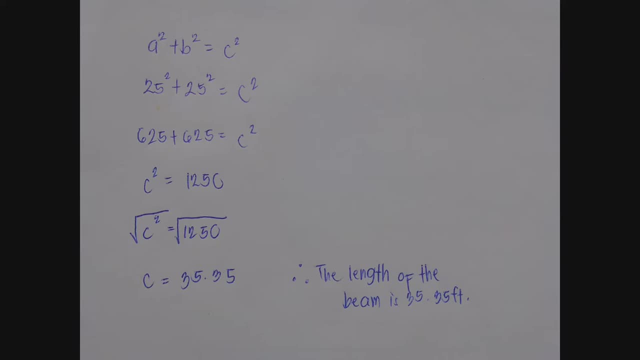 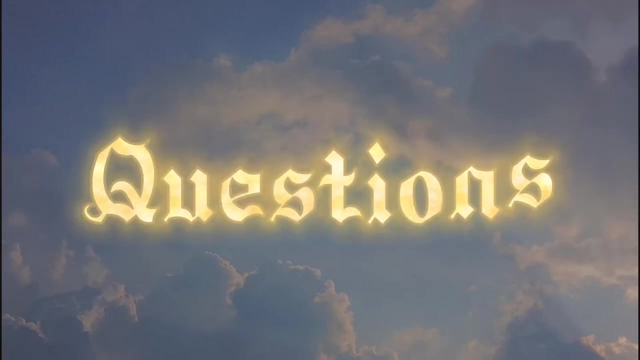 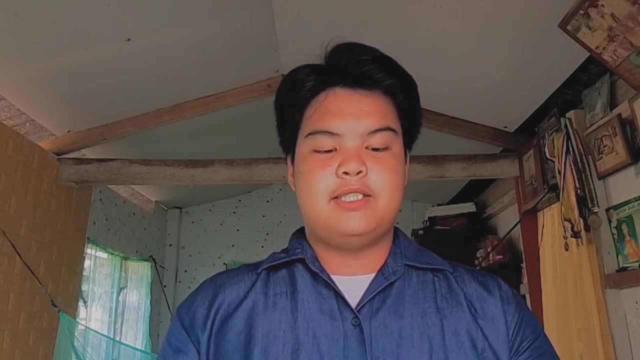 625 plus 625 is equal to 1250.. Square root 1250 is 35.35.. Therefore the length of the beam is 35.35 feet. Question number 1.. Do you think the Pythagorean theorem has been useful to humanity since Pythagoras learned about it? 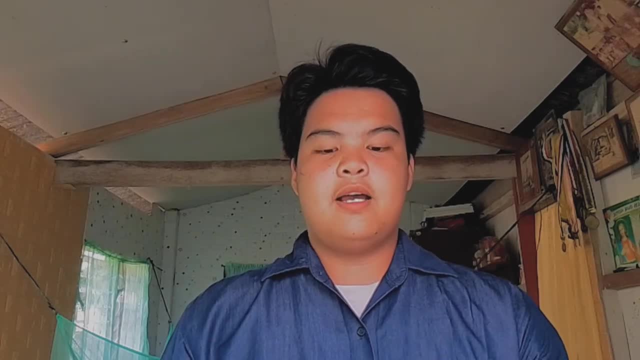 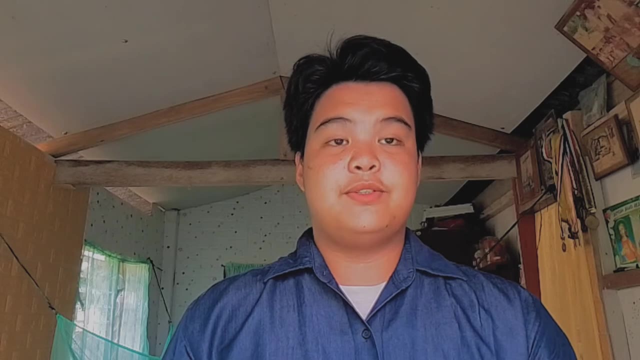 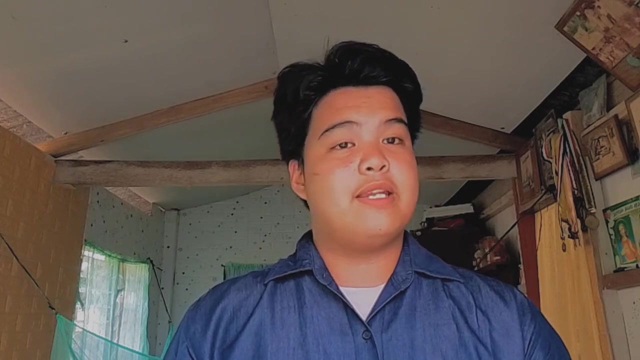 Explain your answer? Yes, As what I have seen and observed from the past until now, Pythagorean theorem is very useful for construction and for navigation. It helps us to know the exact measurement of a thing or an area And to know which way is the fast way to go into your destination. 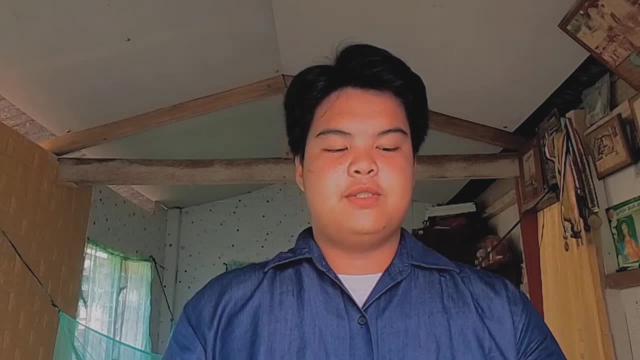 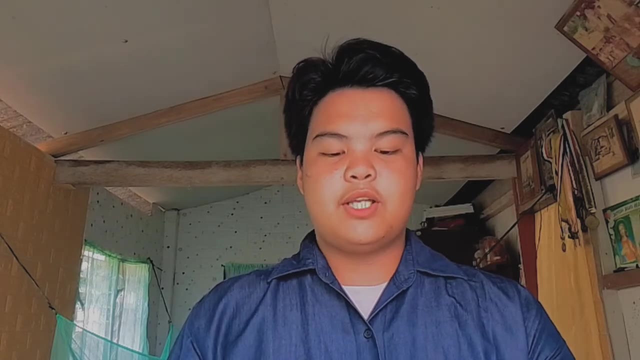 Question number 2.. In your personal life, was there a time that you could have used the Pythagorean theorem? Yes, Most of the time, like knowing shortcuts to go to school and also when you draw or paint and knowing the exact measurement of a thing or an area. Pythagorean theorem is very important to our life. 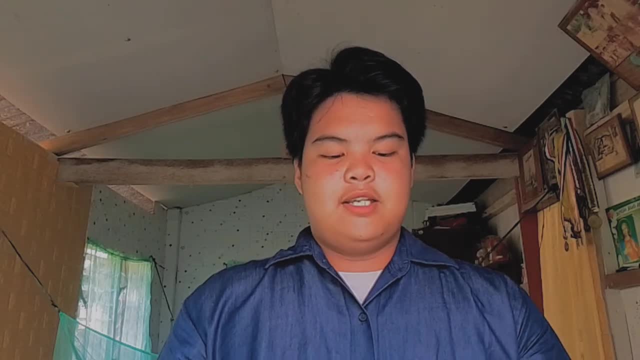 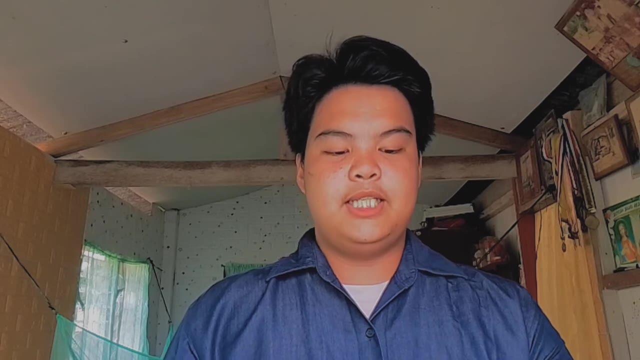 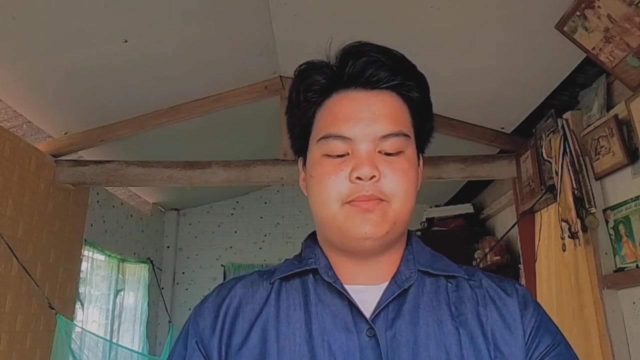 Question number 3.. In general, is it necessary to learn stuff such as Pythagorean theorem? Yes, Because we need and we use it in our everyday life. Every one of us knows Pythagorean theorem is the most important theorem in the whole world.